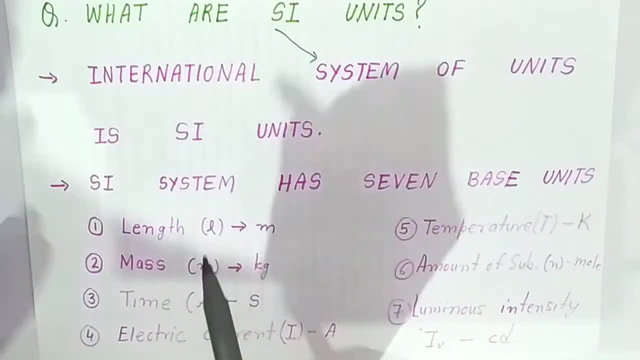 SI unit. SI system has seven basic unit students. In SI system we are going to see the seven basic physical unit. that is length, we are measuring meter. mass, we are measuring the weight. we are showing small m, that we are measuring kilogram. time we are measuring. 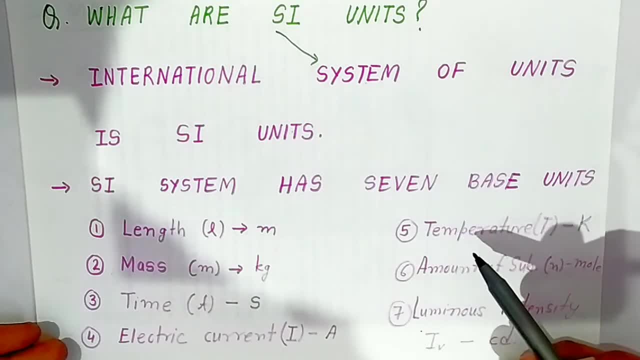 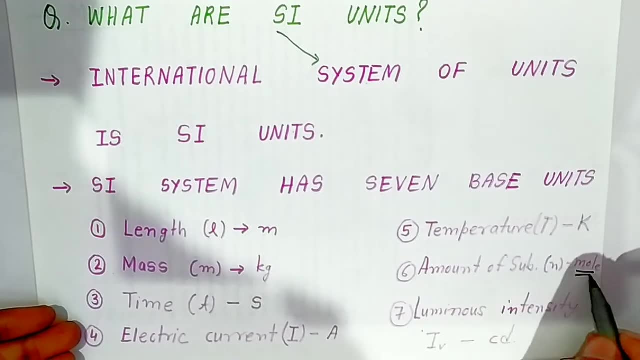 second, electric current. we are measuring ampere. fifth physical unit is temperature. we are measuring in Kelvin, that is capital K, amount of substance. we are measuring mole and luminous intensity. students, we are measuring is cadela, we are showing with CD. So these are the seven. 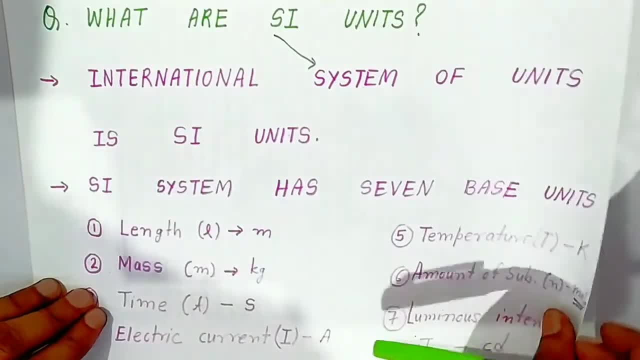 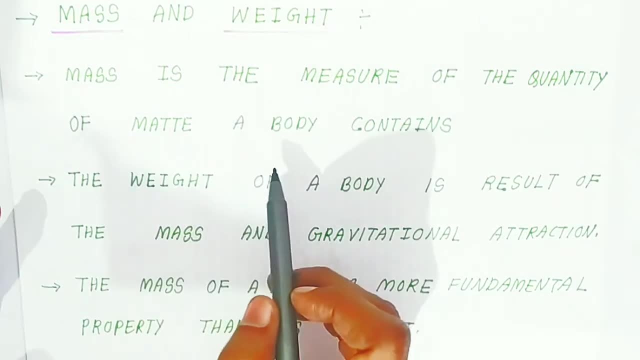 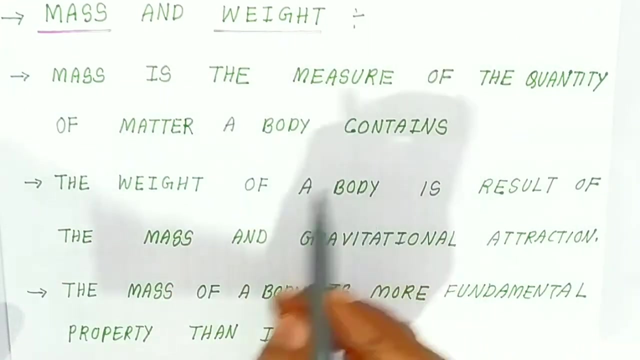 basic SI units, students, that we are going to see in detail Now. students, first students. we should know that. what is mass and what is the difference in weight, Students? mass is the measure of quantity of matter. How many matter are present. matter of a body contains is called as mass. The weight of 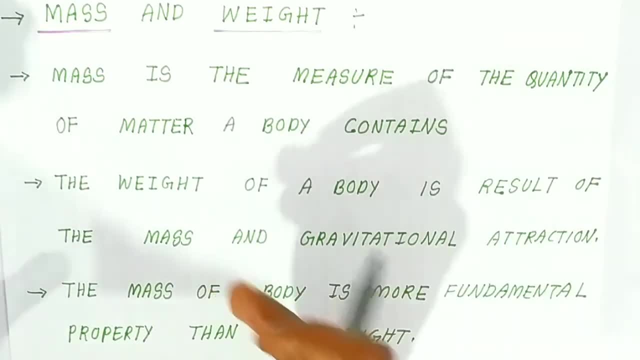 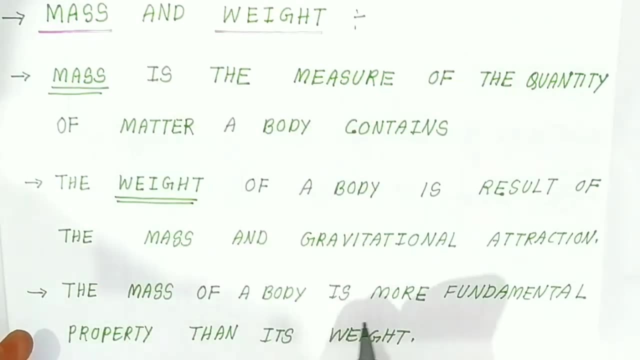 body is result of the mass and gravitation. Mass as well as gravity, both coming together. we call as what Weight? So this is the difference in mass as well as in weight. Students, mass of a body is more fundamental property than its weight. Understand, students, mass will. 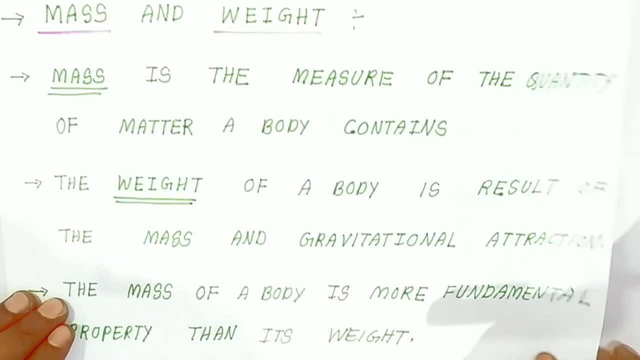 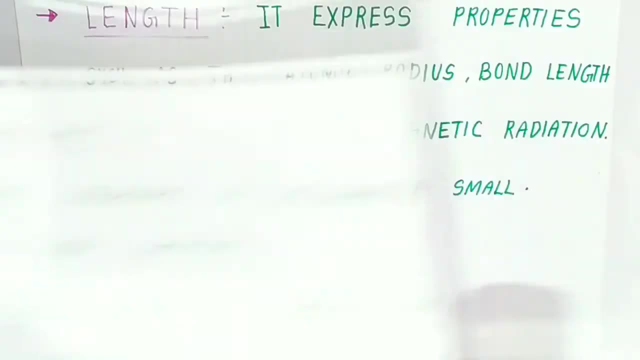 never change in any place, but weight will change because of the gravity. So this is the difference in mass and weight. Students, this you know. you should know from seventh standard. what is the mass and weight? We are learning in eleventh standard Now. students length students, second physical. 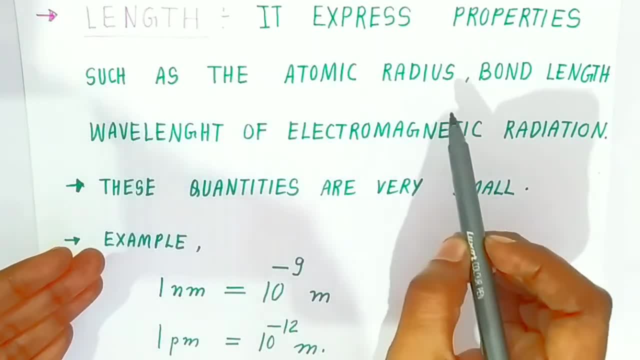 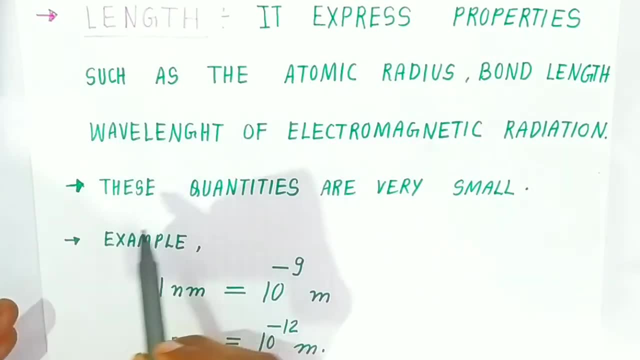 property, students, we are going to see length. It's express property, such as atomic radius. Small is small. what is the length of that Atomic radius bond length, wavelength of electromagnetic radiations that we are going to measure? These quantities are very small. 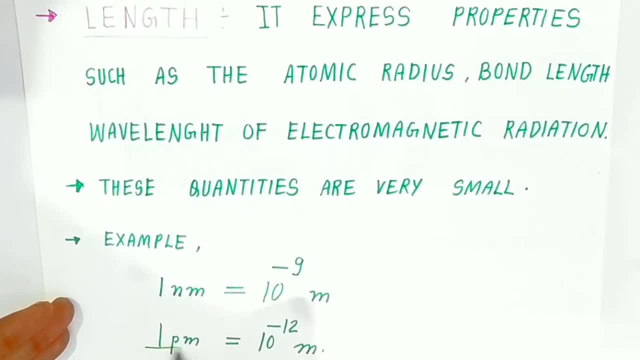 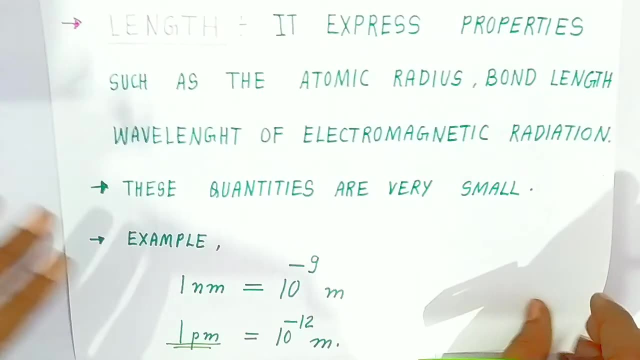 students, one nanometer equals to ten is to minus nine meter, and one picometer equals to minus ten is to minus twelve meter. So these are the very, very small quantity that we are going to measure the atomic radius, bond length and wavelength. So this is the 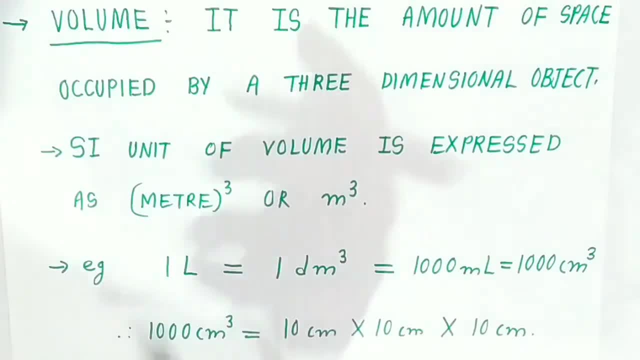 second, physical properties. we are going to see that, students. we are going to see the volume. it is the amount of space occupied by a three dimensional object. measuring cylinder, students. it measure the volume. so it is the three dimensional object. si unit of volume is expressed in meter cube. si unit is volume we are measuring in meter. 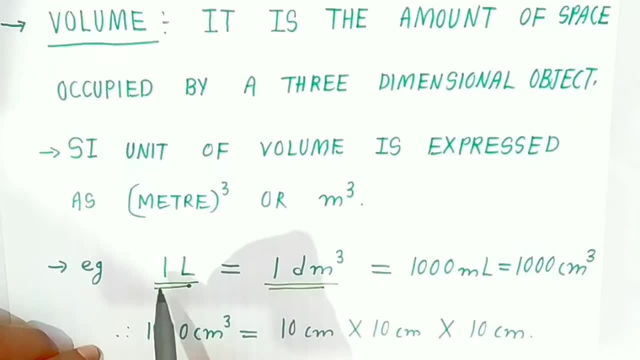 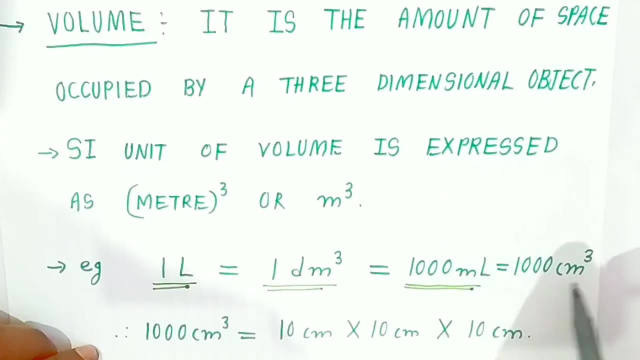 cube one liter. i mean we can write one dm cube. one liter is equal to one dm cube because dm dm is three dimensional object, that is equals to thousand ml. a thousand ml you also call as centimeter cube. okay, students, for liter students, we are using what dm cube for centimeter milliliter. 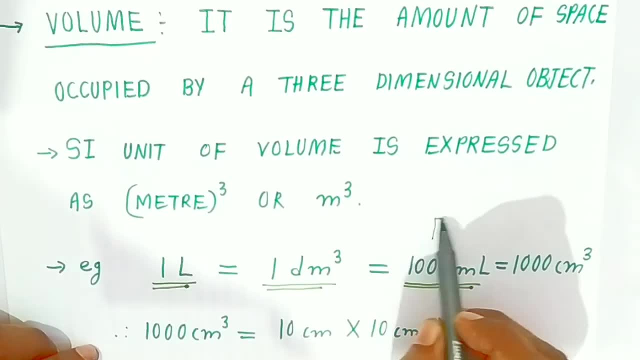 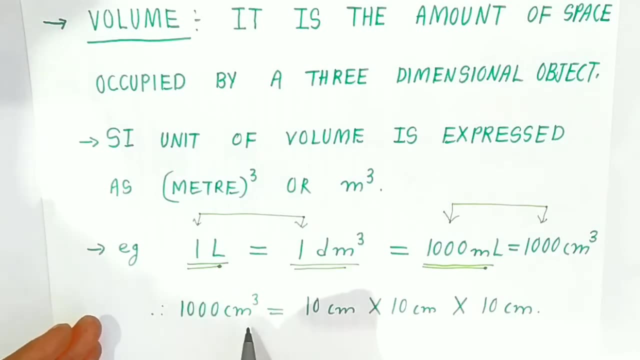 we are using centimeter cube students, understanding both the quantities are same: thousand thousand. we are one and one okay students. so these are the about the volume. hundred one thousand centimeter is equals to length, breadth and height. this is length, breadth and this is what height, okay. 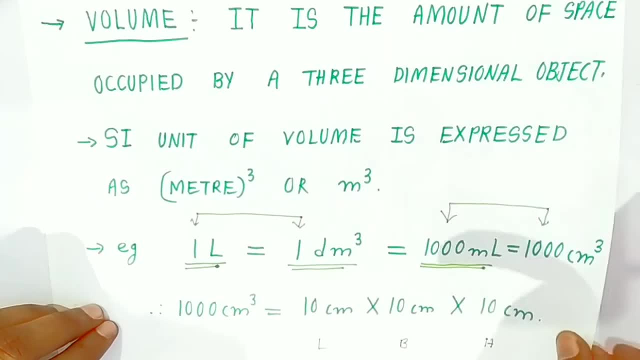 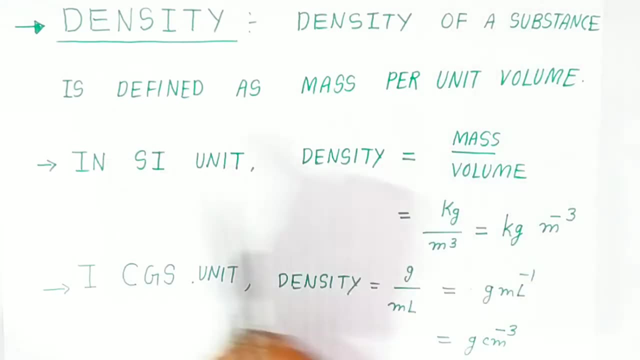 students. so this way we have called. that is why we call a three dimensional object. now, after that distance from volume, we are going to see. density of a substance is defined as mass per unit volume. mass upon volume is called as density. this si unit is one kilogram per meter cube, this minus. 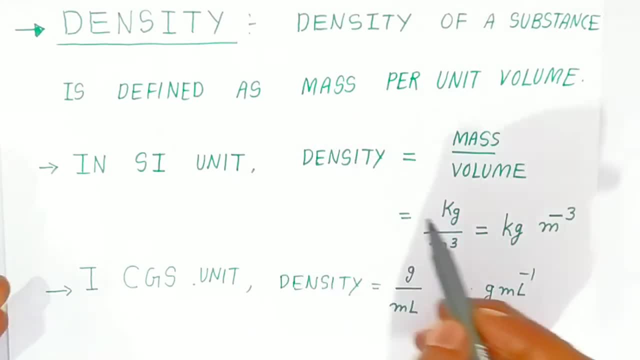 we are going to see. the density of a substance is defined as mass per unit volume, mass upon volume. we can say what per per meter cube, kilogram per meter cube, is the si unit of density. students, mind well, when you are in cgs, unit students, gram per centimeter cube per student, because this minus is 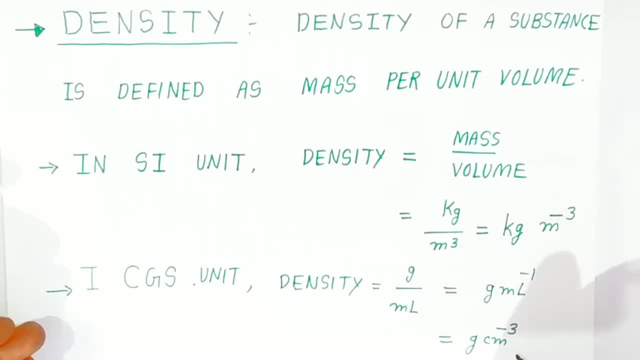 saying that means this centimeter is in denominator. okay, students, this is a gram per centimeter cube, a gram per ml. this is understanding, students. these are the very important units of density. density of substance defined as mass per unit volume: how much dense substance is there this way? 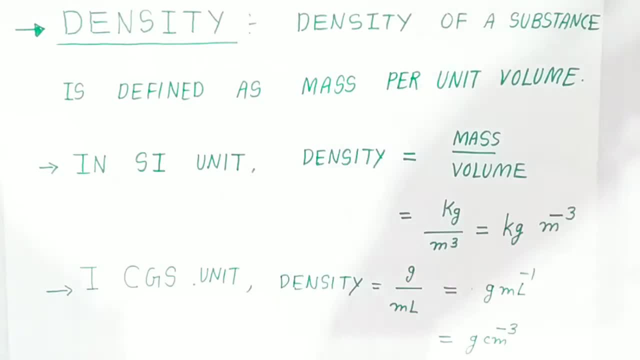 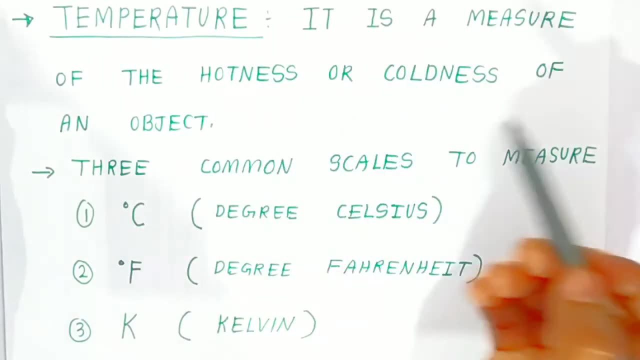 you can. with the help of this formula, we can comes to the density of the substance. now, students, after knowing the density, students makes physical properties. temperature. temperature is students. it measure the hotness and coldness of the object. how much hotness and cold the substance is with the 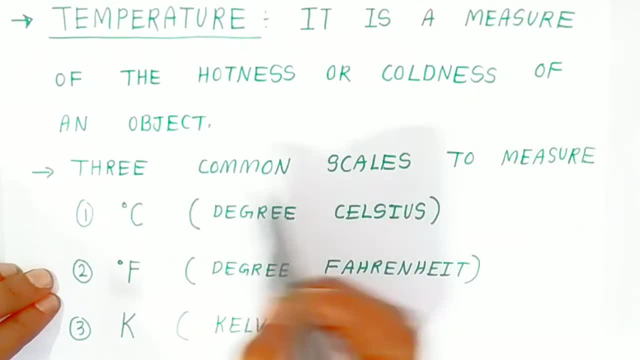 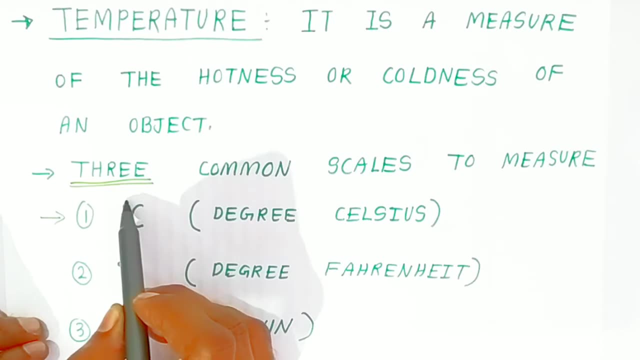 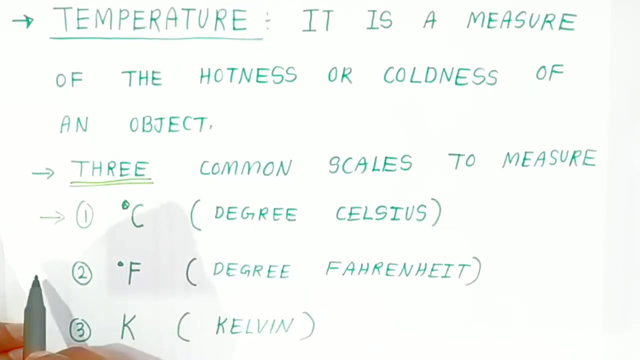 help of the temperature. now, students, generally students: three common skills. of the three common skills we are using for to measure the temperature first, students. first is degree celsius. this, this is the called as degree celsius. c stands for celsius and this zero is one degree. after that is one second. uh scales. we are you going to measure temperature? 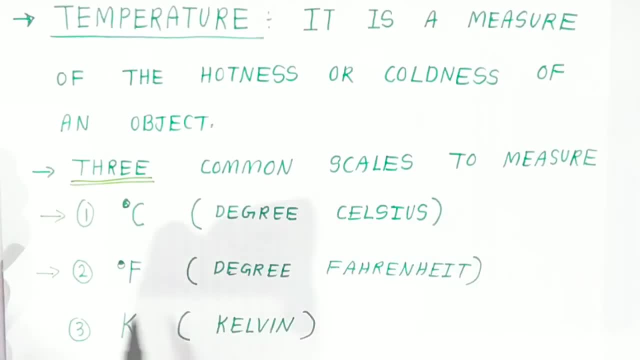 is called as degree fahrenheit because the fahrenheit is scientist name, same way celsius was the name of the scientists because they have discovered. so we call it degree celsius, which is called a degree fahrenheit. and here we are not using degree, we are using only kelvin k. 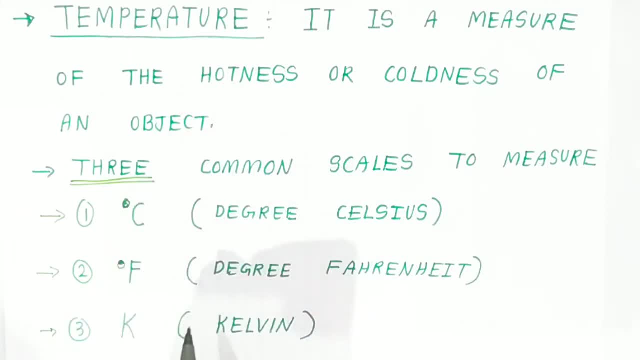 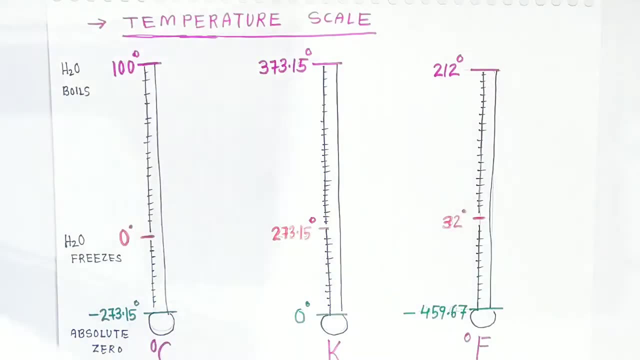 we are not going to put the zero symbol. so this is called as three scales to measure the temperature. students. the first one is degree celsius, degree fahrenheit and kelvin. now students, after knowing the definition of temperature students, now we are going to see that all three degree celsius degree. 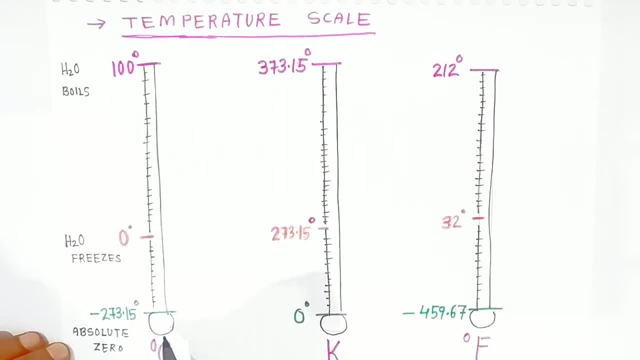 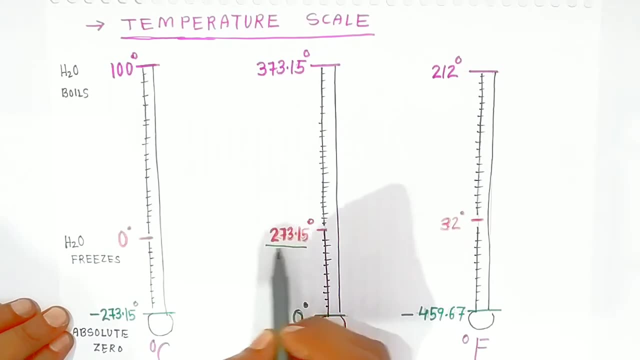 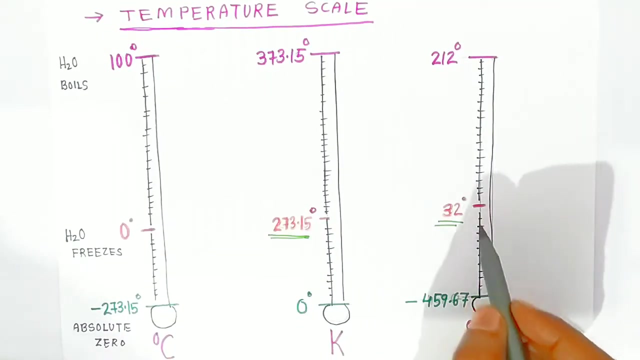 fahrenheit and kelvin. so students, if that um students, you know, water freezes zero degree celsius, same. when it comes to the kelvin students, the same water will freeze at 273.15 degree celsius and same students water freeze will be at 32 fahrenheit degree, 32 fahrenheit. this is the 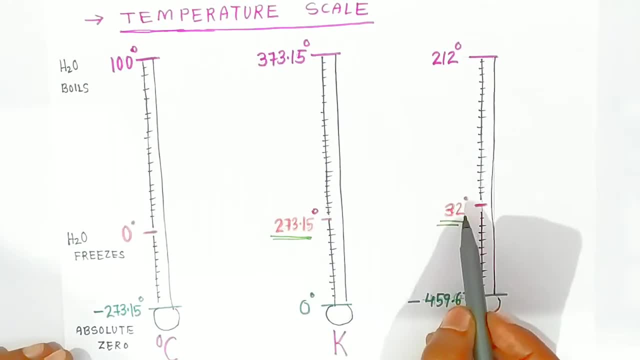 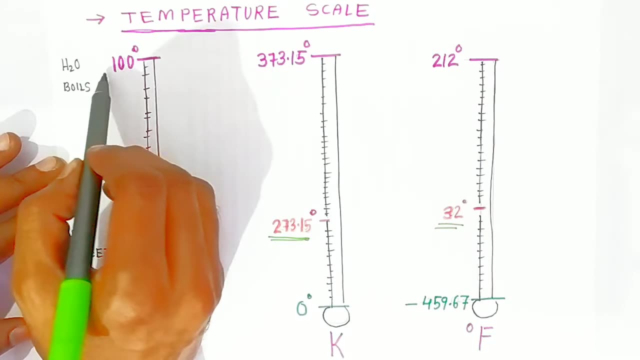 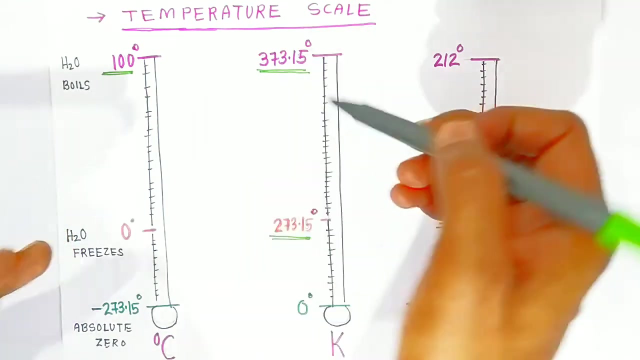 fahrenheit distance, correct distance degree, fahrenheit 32 degrees. so these are the freezing point of in all the three scales. now students, same water students, it boils at 100 degree celsius, so that means in kelvin we can say 370, 3.15 degree celsius degree degree because it is a kelvin. so 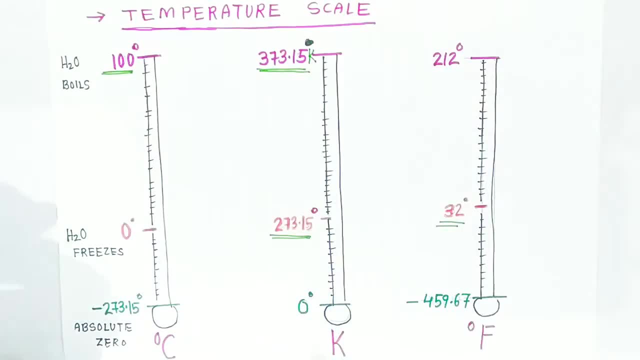 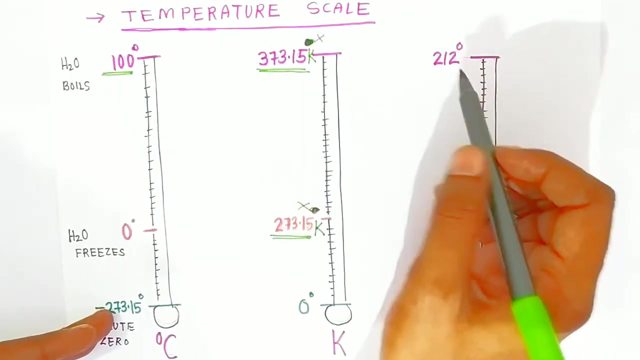 we can. we cannot put zero here. we can put what k? kelvin 370, 3.15 kelvin, okay students. we cannot put this degree. we can put kelvin k, okay students. so this we cannot put here. so we are putting only kelvin. when you are using in fahrenheit distance, the water boils at 212 fahrenheit degree fahrenheit. 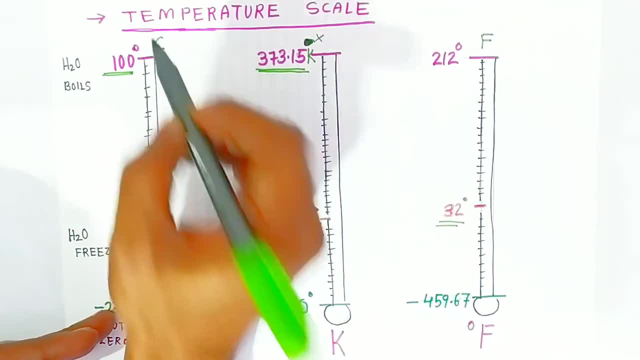 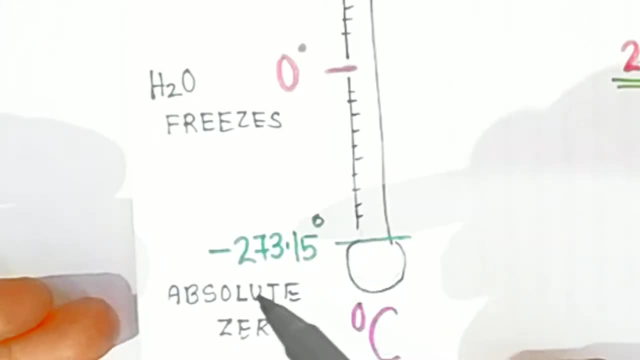 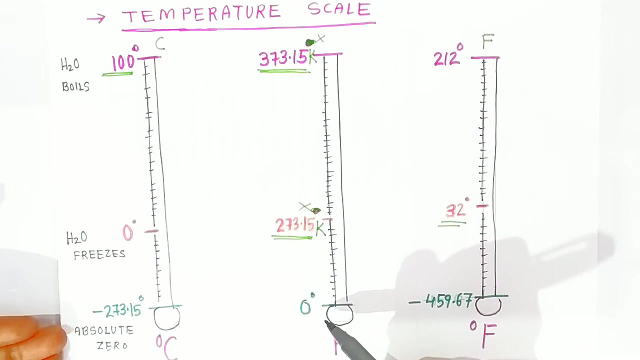 degree, because it is fahrenheit, okay, and this is kelvin, and this is what degree, celsius, okay, students. so this is the way. now here, students below absolute zero students, what we call as minus 273.15 degree celsius is called as absolute zero. now here, zero kelvin. we called as what? 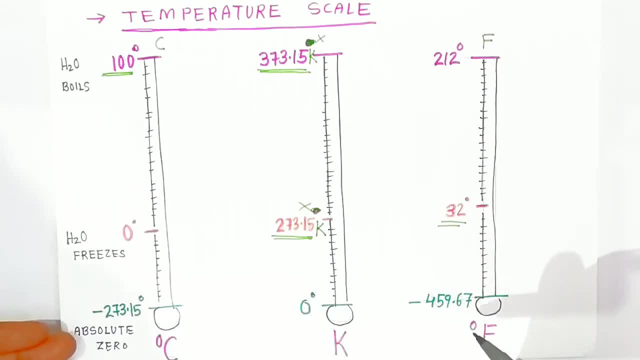 absolute zero. now here students in fahrenheit, degree fahrenheit minus 459.67 fahrenheit a degree fahrenheit. we called as what? absolute zero. so these are the three scales we have have seen. absolute zero, that means water freezes at zero degree celsius and 100 degree celsius. 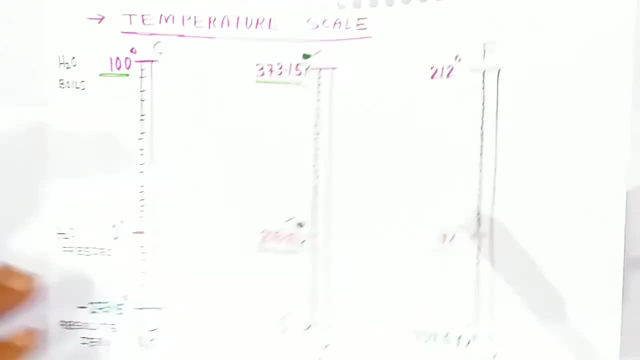 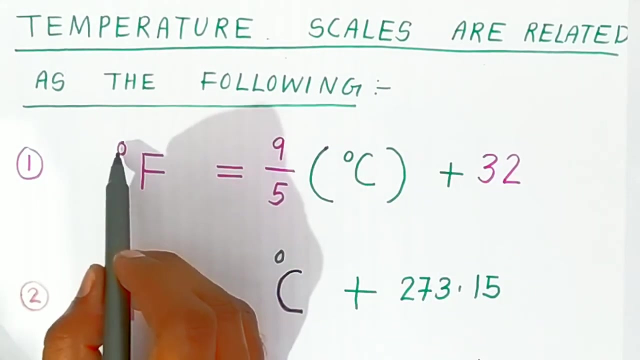 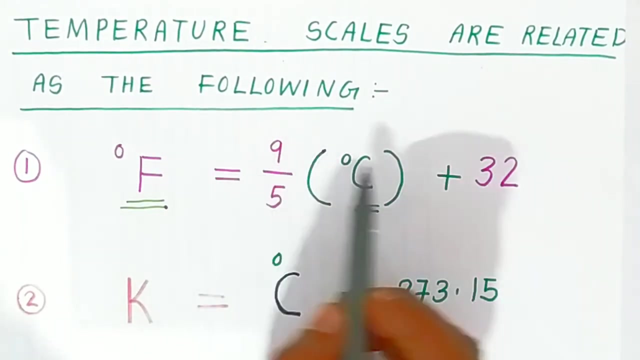 in all three scales. now, students- these are very important students. now, after that, students: the temperature scales are related as the following: all the three scales how they are going to relate distance: this is the degree fahrenheit, distance, degree fahrenheit and degree celsius: how they are related. one degree fahrenheit is equals to 9 upon 5 times degree celsius plus 32. this we have. 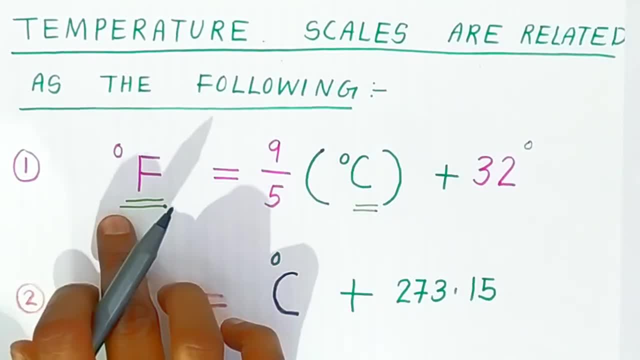 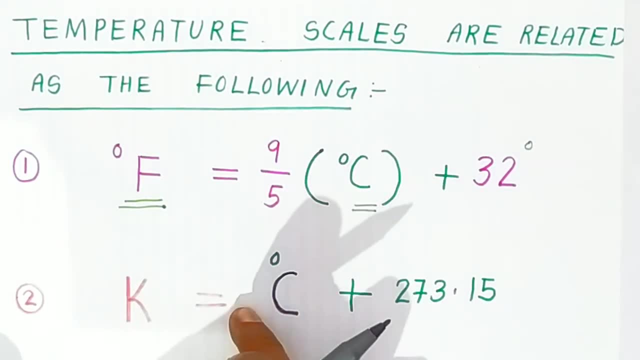 to add. okay, students, so this is one fahrenheit is equals to 9 upon 5 degree celsius plus 32. now one kelvin is also equals to this. kelvin is equals to 1 celsius. we are adding 273.1 degree. so this is the about the how you are going to convert kelvin into degree, celsius and degree.